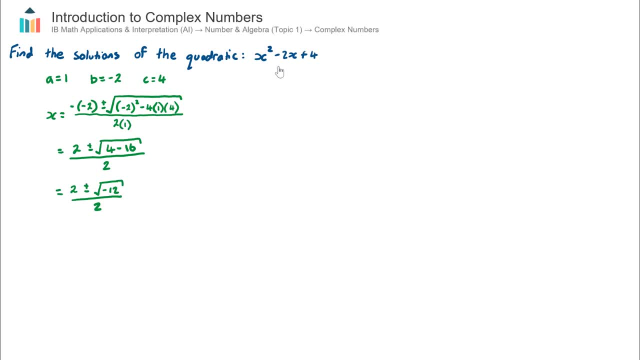 and usually as a last resort, it would be using the quadratic formula, which is what I have started off here. So I substituted in my values for a, b and c, did some working and I got to this point here and I thought: oh no, I can't proceed any further. I have the square root of a negative number. 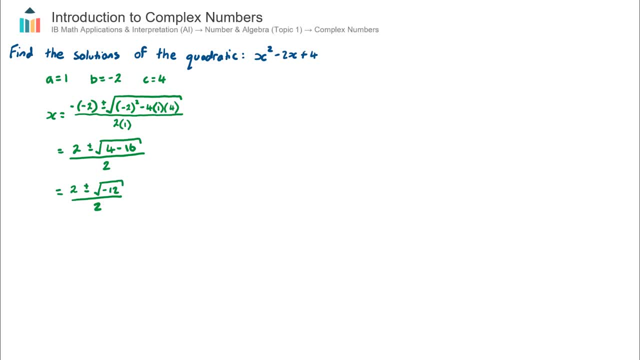 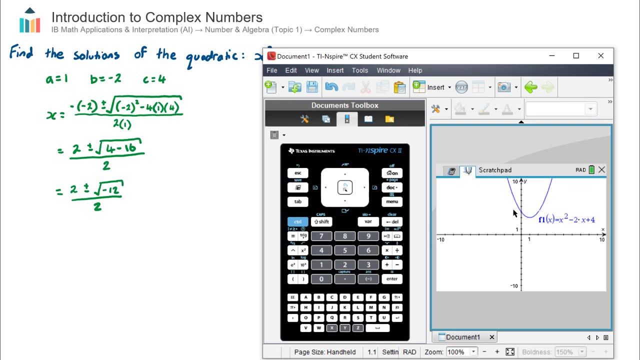 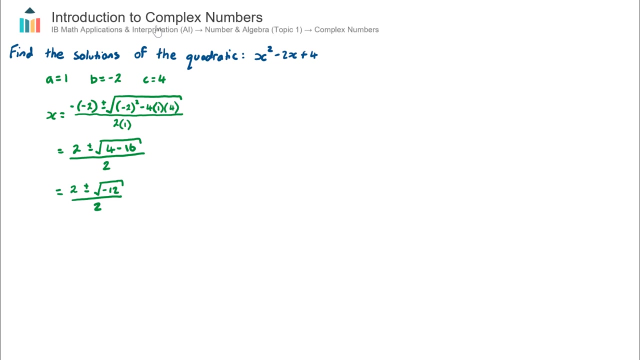 therefore, my quadratic does not have any real solution. And if I was to visualize the quadratic, that is indeed the case. it does not cut through the x-axis. therefore, it does not have any real solutions. So we would usually stop at this point here. however, if we, if we now introduce complex numbers and how to deal with the square, 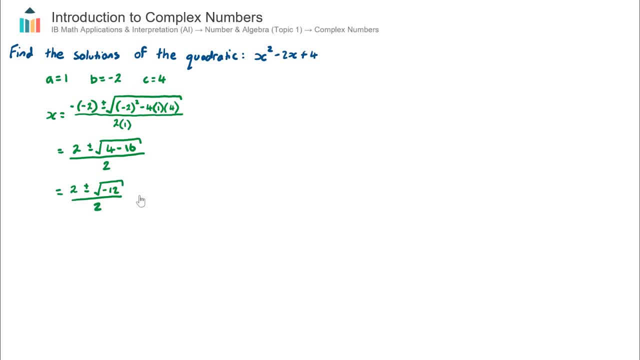 root of negative numbers. we can actually take this further and find the complex roots of this quadratic. So let's go ahead and do this and then, during this process, you'll start to see what an imaginary number is, which is how to deal with the square root of a negative number. 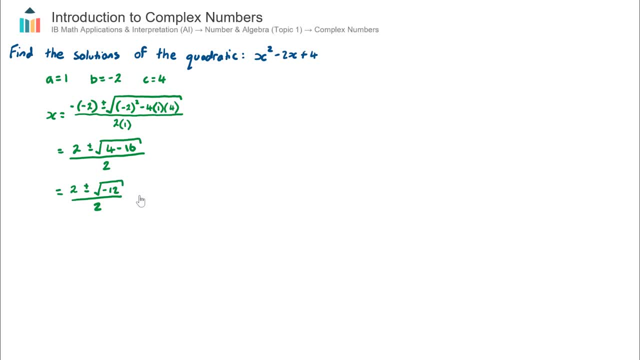 And then at the end, what a complex number is in Cartesian form. So let's go ahead and do this. I need to deal with the square root of negative 12, so I'm going to split the negative 12 up into three factors of negative 12 and I'm going to choose 4, 3 and negative 1, and I wanted to do it in this way. 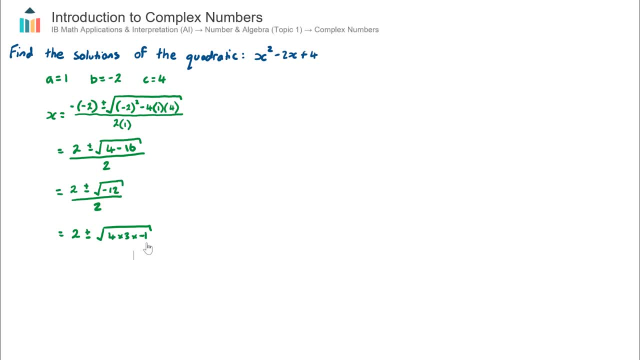 because I want the square root of negative 1, because that allowed me to replace that by this new number, i, which stands for an imaginary number. So I'm going to split the square root of negative 1 and negative 2, and I'm going to do that by using the square root of negative 1 and negative 2.. 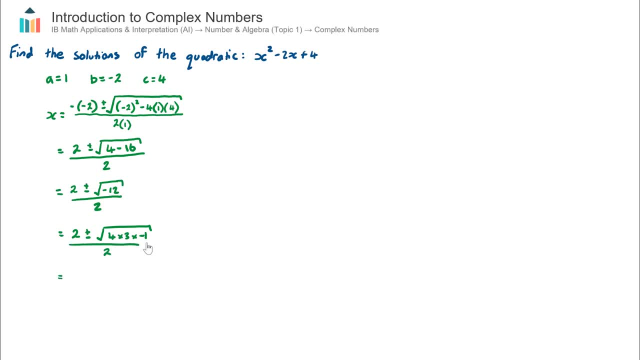 So this is still all over 2.. Now, using my knowledge of surds, I can actually break up these three factors that are all under the same square root sign into three individual surds. So this will become 2 plus or minus square root 4 multiplied by square root 3 multiplied by square root of. 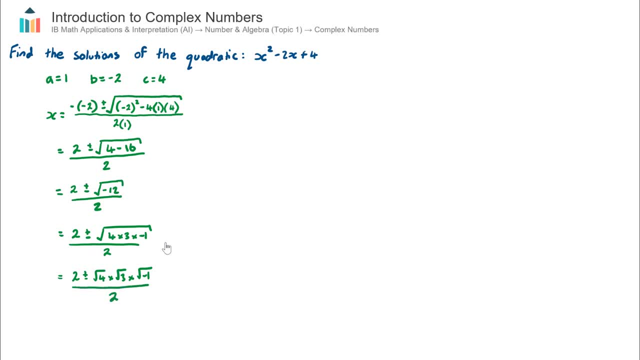 negative 1 over 2.. Now I know that the square root of 4 is 2. I'm going to leave the square root of 3 as is and the square root of negative number. here's where we introduce this new number, here, this new 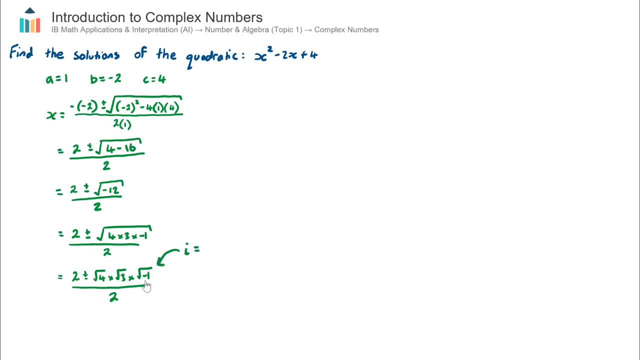 number i. i stands for an imaginary number and where i is the square root of negative 1.. So now we can deal with square roots of negative numbers because we can replace it with this imaginary number i. So if I take this one step further, this will be 2 plus or minus. now root 4 is just 2. 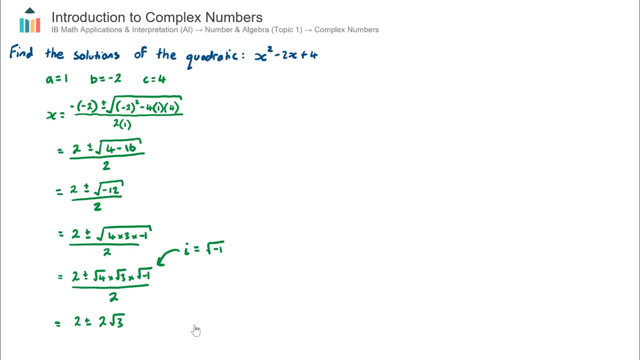 root 3 I'm going to leave as is as root 3, and the square root of negative 1 I'm going to replace with all over 2.. Now, if I look at this, here, there's 2, root 3, i. sometimes the i is written in between. 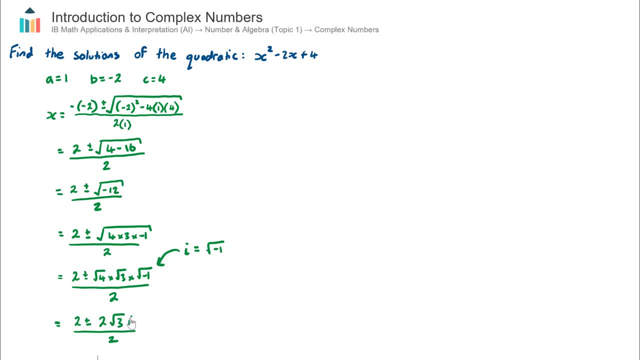 the 2 and the root 3.. I tend to like to leave it at the end, but some textbooks will have this as 2 i root 3.. I can actually simplify this one step further. now. looking at it, I can divide both the numerator and the denominator of this fraction by a common factor, 2.. So that leaves me with a nice 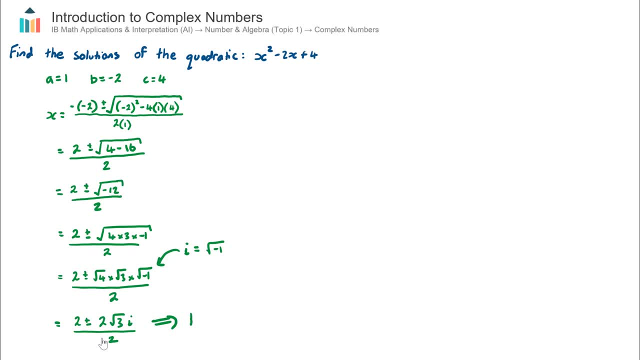 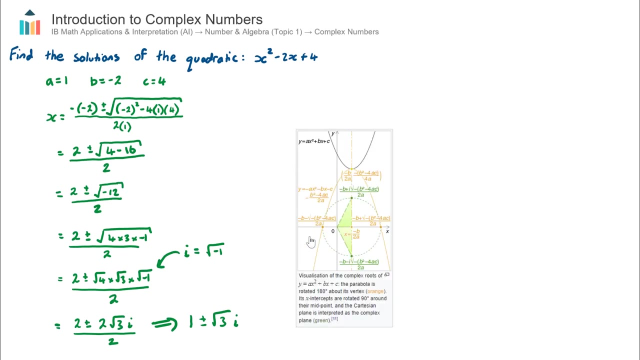 simple, and what I'm about to write here is called a complex number: 1 plus or minus, root 3: i. and it's a complex number because it has an imaginary component. Part of the number is attached to this imaginary number i. Now, if you're wondering what these roots look like, it's a very good. 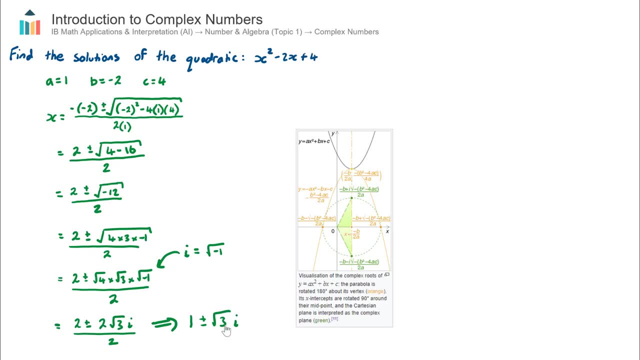 question. It's called an imaginary number here because it's not. I can't actually point to it. on the real number line, Wikipedia has a nice diagram here of what the complex roots of a quadratic looks like if you try to imagine it or visualize it. So this black line here is a quadratic. it 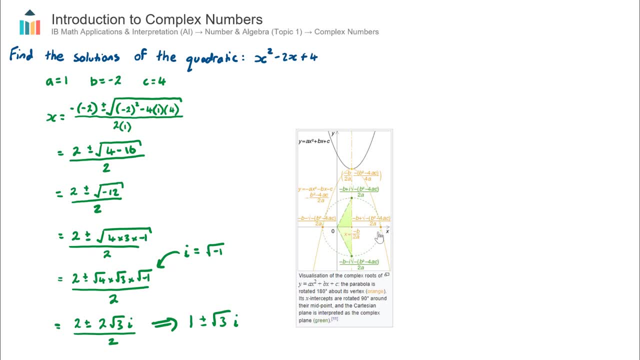 sits above the x-axis. so there's no real solutions and the complex solutions will be this orange line here, which is kind of a reflection, a horizontal reflection about the turning point. Now I won't go into too much detail here, because feel free to go and read this article just by searching. 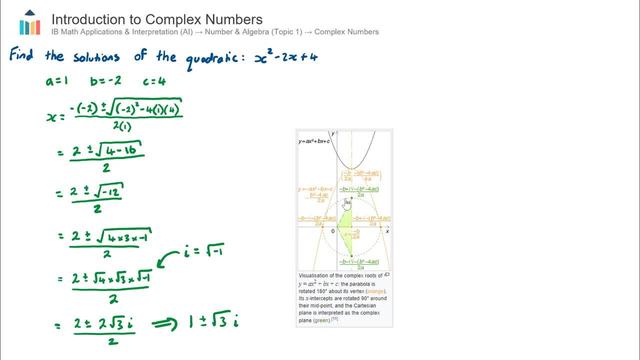 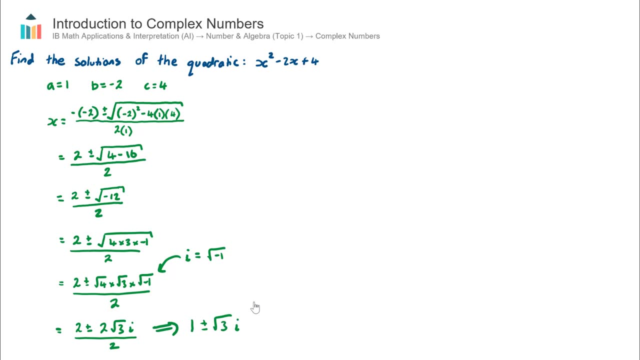 quadratic equation- wikipedia. but if I was to drill into the explanation of this, that would take me quite a long time, so I'll leave that for you to read up on. Okay, but let's now summarize what we have covered so far. We have introduced this new type of number here, and this actually completes a number. 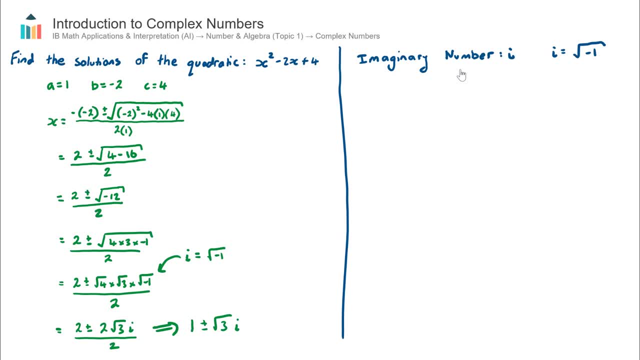 systems. so our number system was positive integers, all integers, real numbers, irrational numbers, and this is actually the last part of that. now, imaginary numbers: i, and this allows us to deal with the square root of negative number, where i is defined as the 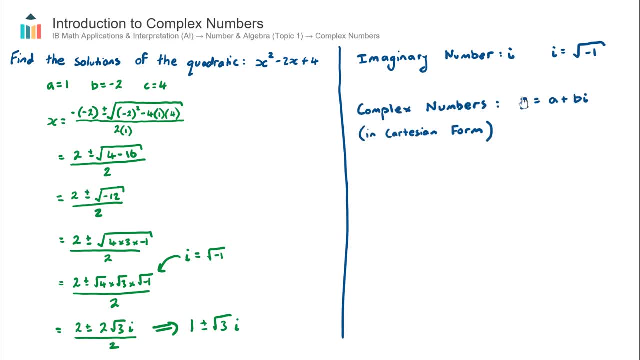 square root of negative one. We have also introduced what a complex number is, which is in Cartesian form, which is one of the three forms of complex numbers. Let me share, guys. I'm go go down with you a little bit numbers that you'll encounter in your course. I'll cover the other two forms, which is polar and euler. 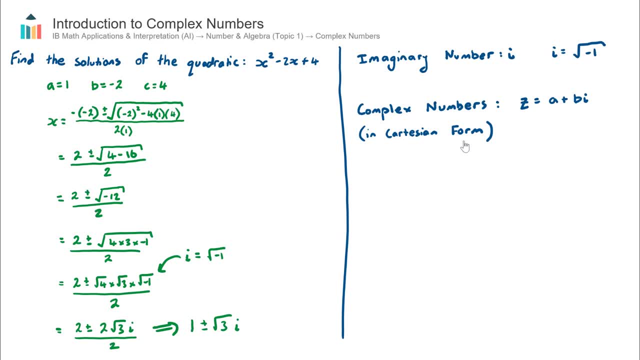 in the next video, but so far we have what a complex number is in Cartesian form. So back to my example here. to start the video I had 1 plus square root 3i, So the form of a complex number in Cartesian form is a plus bi. Now we usually- textbooks and exam papers- will define complex numbers either, as 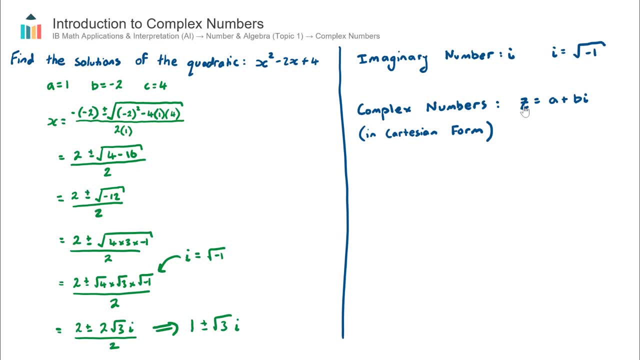 z or w. so I'm just going to use z here. So the complex number in Cartesian form is: z equals a plus bi. So as an example, so let's just do example, let's just say z is equal to, and I'll use this example that I brought down from the first example, I'll just use the positive version of this. So 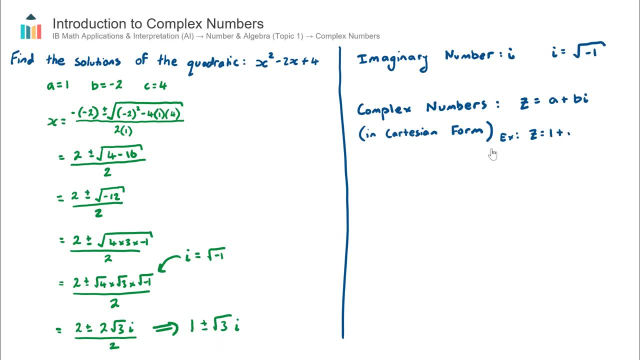 this example will be 1 plus root 3i. Now this complex number here has both real components, which is the 1. There's no i attached to the 1, and also an imaginary component, which is the root 3i, And you can. 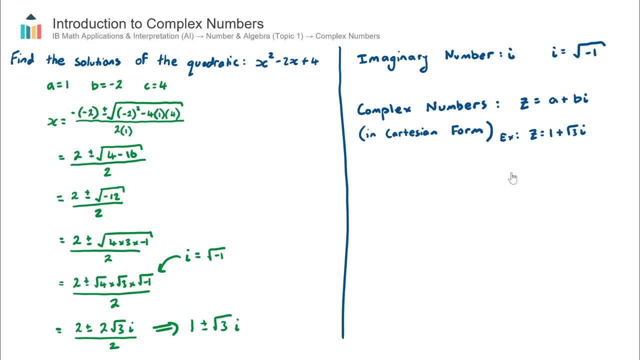 actually write that down. So the proper notation of defining that will be: the real component of my complex number z is equal to 1 and the imaginary component of my complex number z is equal to root 3.. Now the final thing I want to cover in this video is to how to visualize a complex number in 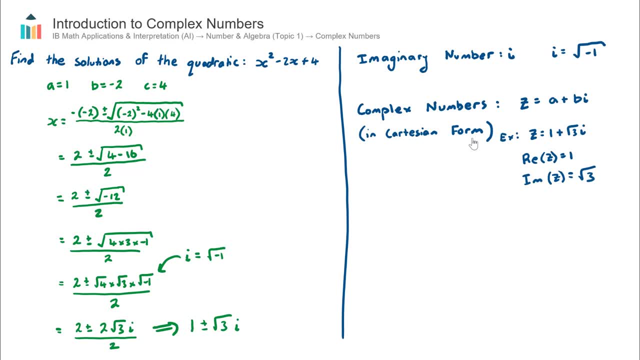 Cartesian form. So I'm going to go ahead and show you how to visualize a complex number in Cartesian form on a complex plane. Now that sounds quite difficult: complex planes and complex numbers- but it's actually not, If you have a sound understanding of coordinate geometry. so how to plot? 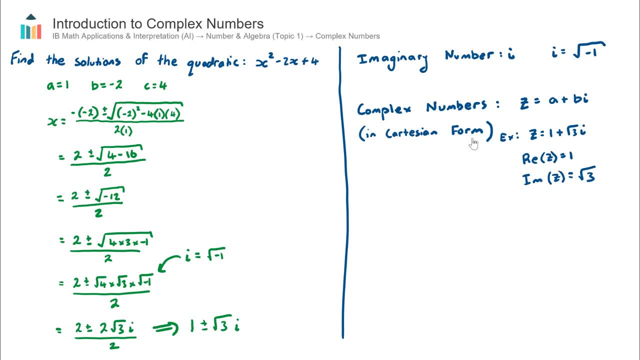 coordinates on an x- y axis. it's about, that's about all it is to it, except it's not. we're no longer going to have an x- y axis, we're actually going to have a real and an imaginary axis. Let's go ahead and visualize that. So this here. so we have this first point here, the second point here, the third. 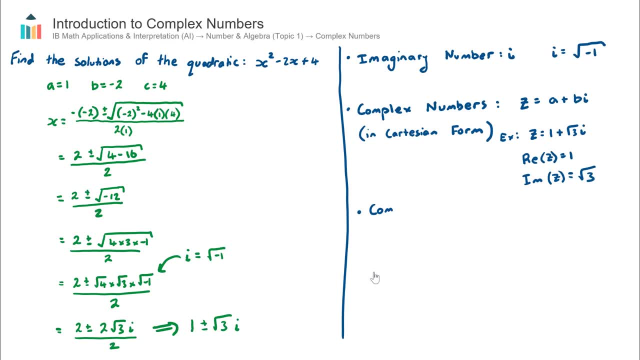 point I want to cover is complex planes. Now, they are also known as argand diagrams, and I actually tend to call them argand diagrams, but the AI documentation actually refers to them as complex planes, Argand diagrams, but they are the same things. Okay, so a complex plane has a horizontal